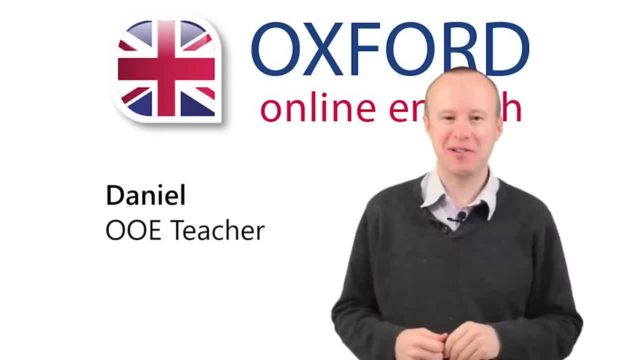 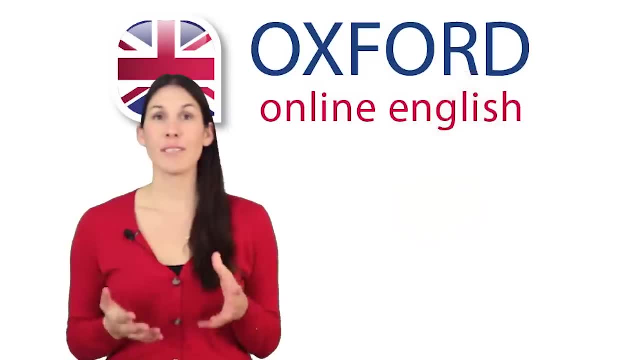 Hi, I'm Daniel. Welcome to Oxford Online English. In this lesson you can learn about using adjectives in English. You'll see basic information about English adjectives, what they do and how you can use them. Then you'll see some more details about different types of adjectives and what 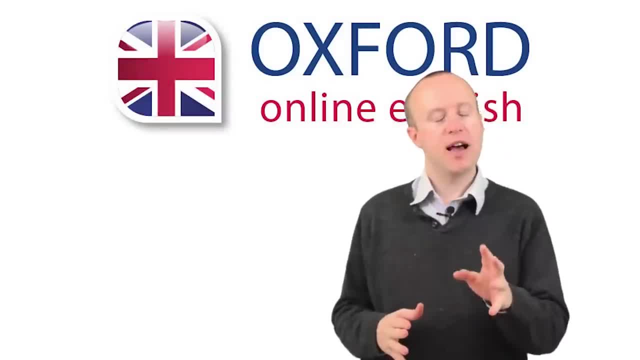 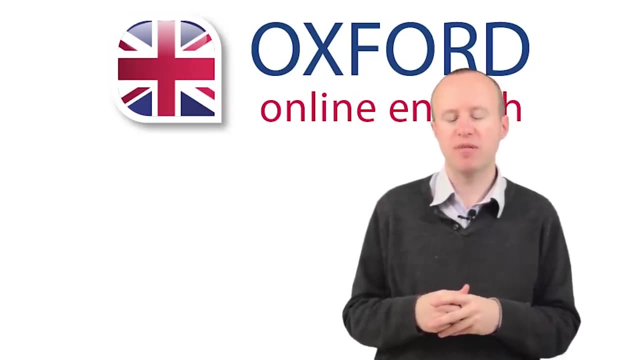 they mean? Before we start, have you visited our website, Oxford Online English dot com, If you want to improve your English? there are free video lessons as well as listening lessons. We also have a large selection of professional teachers who can help you improve your English. 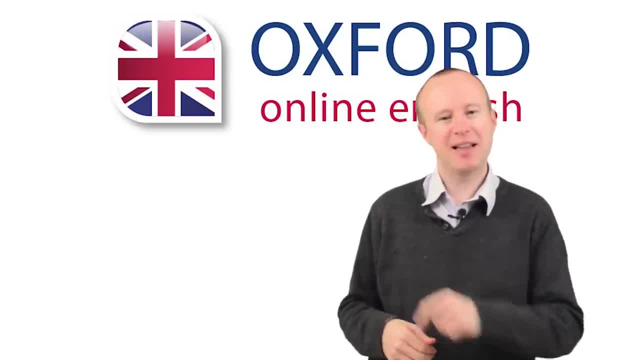 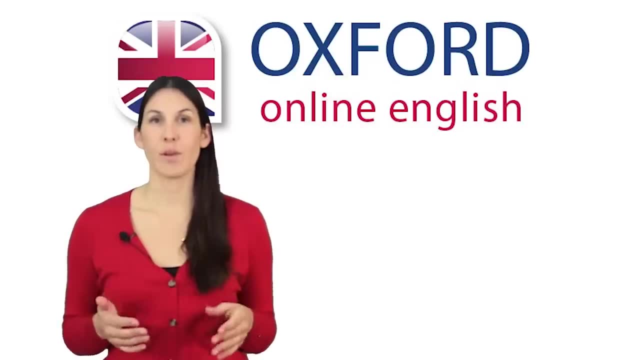 in online classes. But now let's get back to the lesson. First a question: What do adjectives do? Adjectives describe nouns. They add information to a noun or a noun form. Adjectives describe nouns. They add information to a noun or a noun form. They add information to a noun or a noun form. 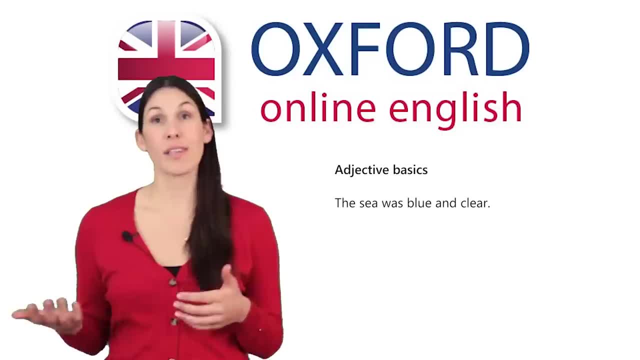 Adjectives describe nouns. They add information to a noun or a noun form. They add information to a noun or a noun form. For example, the sea was blue and clear. The adjectives blue and clear add information to the noun sea. 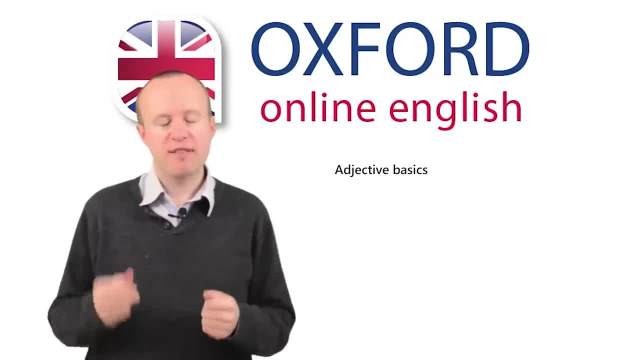 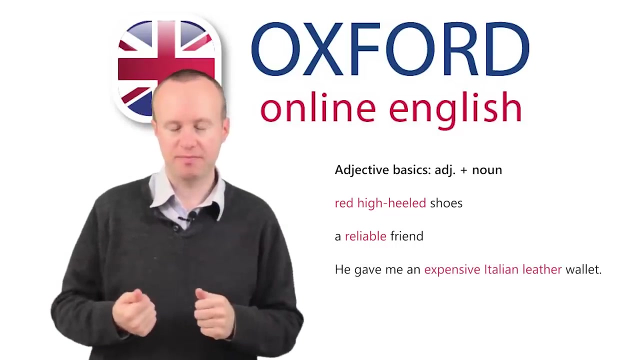 Adjectives can be used in many ways, but there are two common patterns. First, you can put adjectives directly before the noun. they describe, like this Red, high-heeled shoes, A reliable friend. He gave me an expensive Italian leather wallet. 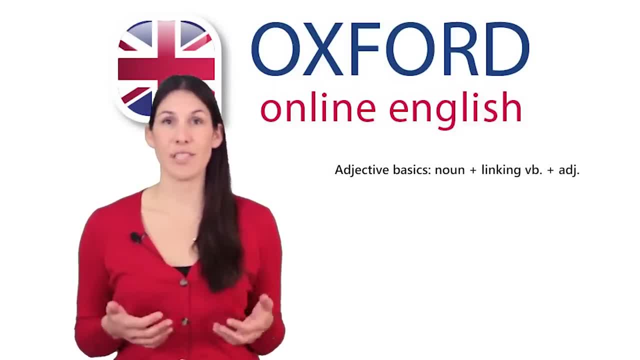 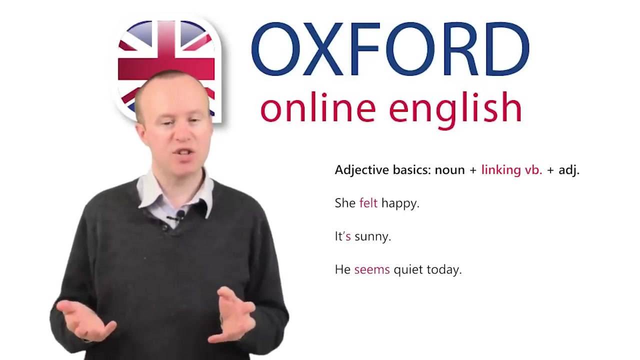 Secondly, you can use a linking verb plus an adjective. after a noun like this, She felt happy, It's sunny. He seems quiet today, By the way. what are linking verbs? Linking verbs add information to a subject. Common linking verbs include be, seem, become, feel and appear, although there are many others. 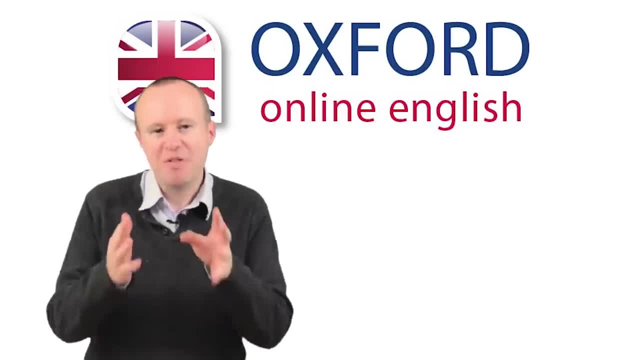 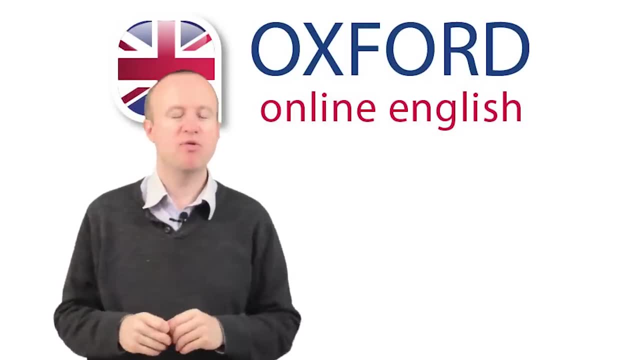 You don't need to worry about this right now. Remember the basic point – adjectives can go before a noun or after it. This will become more important later in the lesson. Keep watching to find out why. Here's another question for you. 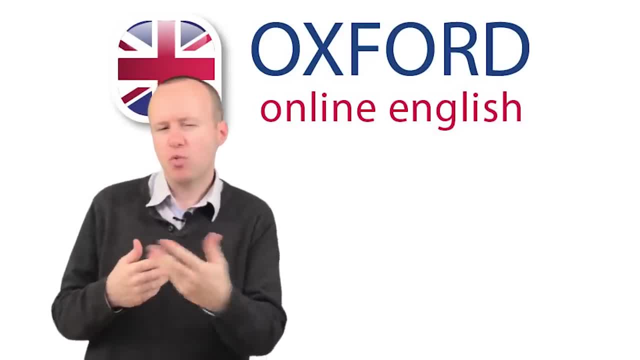 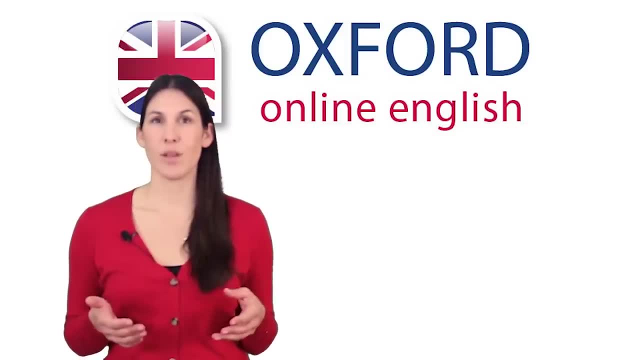 How can you find the adjectives in a sentence? What do adjectives look like? There's no simple answer to this question. With all parts of speech, it's better to look at full sentences and think about context and meaning. Let's do a quick test. 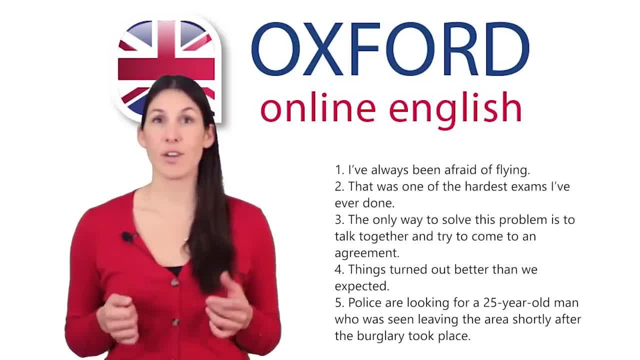 Here are five sentences. Can you find the adjective or adjectives in each one? Pause the video if you need more time to think. You'll see the answers in a few seconds Ready. Here are the answers. You can see a few useful points here. 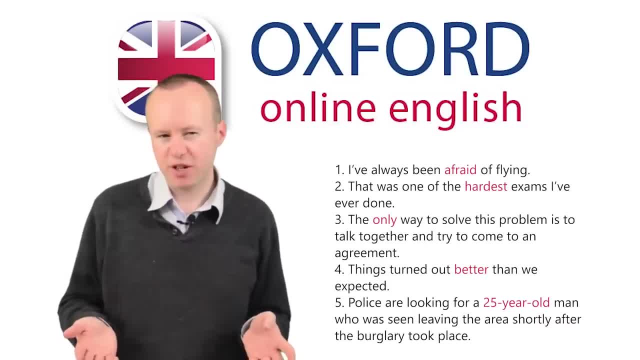 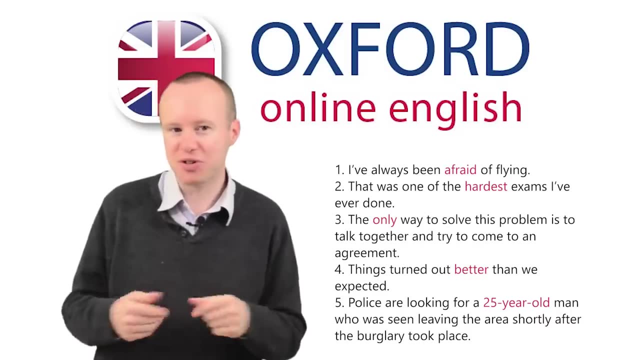 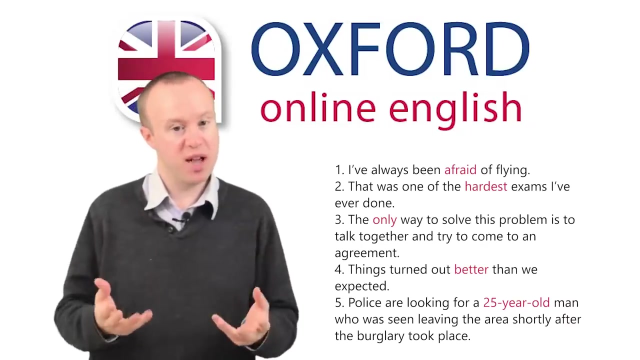 Firstly, adjectives don't look similar to each other. Adjectives can have many different endings, and they can even end with –ly, like most adverbs do. Secondly, adjectives also have different forms. For example, many adjectives have comparative forms like good, better or superlative forms. 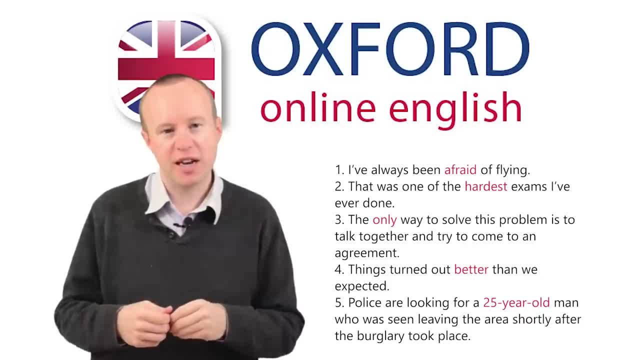 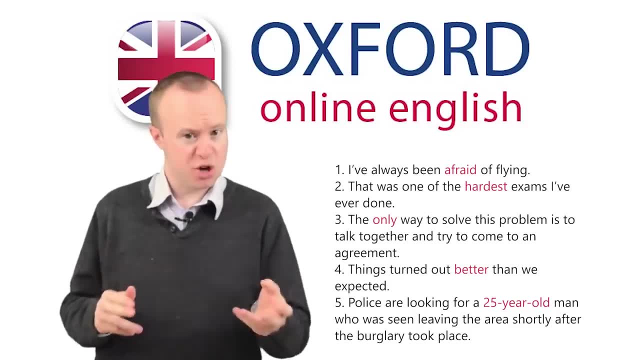 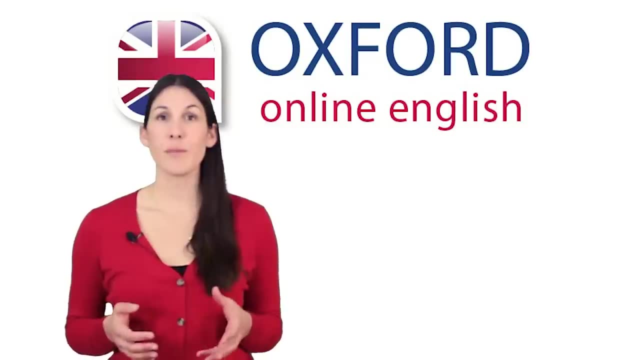 like hard hardest. Thirdly, some adjectives are compound meaning. they're made from two or more other words. This is common with numbers, as in a twenty-five-year-old man. Now you know some of the basics about adjectives and how to use them. 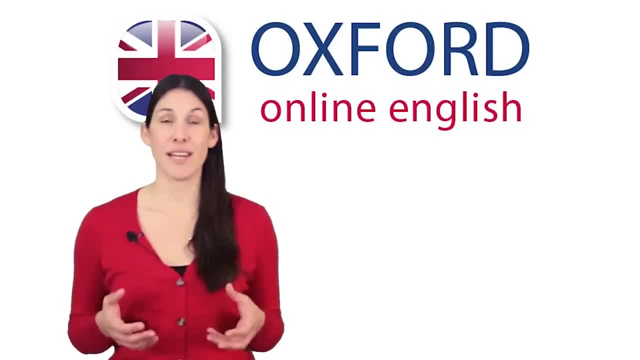 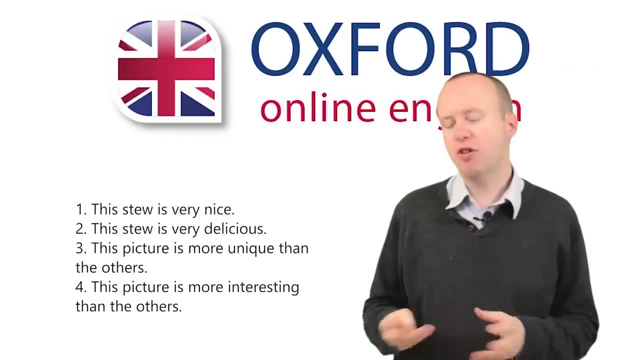 Let's go into more detail in a moment. Let's go into more detail about different types of adjectives. Look at four sentences. Two are right and two are wrong. Can you see which sentences are correct? Do you know why the other two sentences are incorrect? 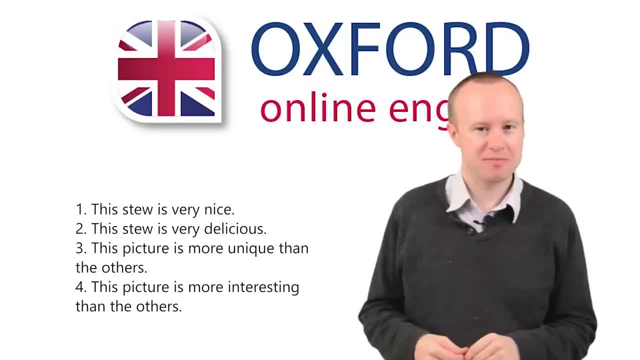 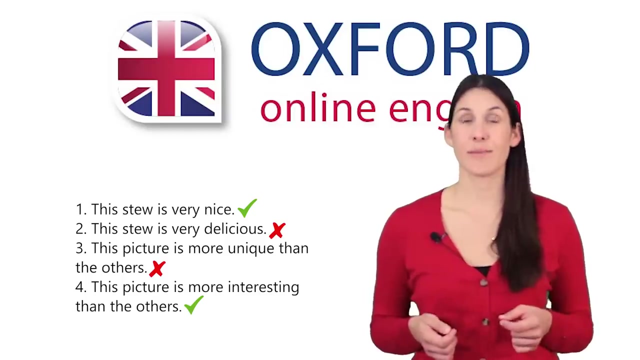 Pause the video if you need more time to think about it. Ready, Let's look together. Sentences one and four are correct. Two and three are incorrect. Did you get the right answers And can you explain why sentences two and three are incorrect? 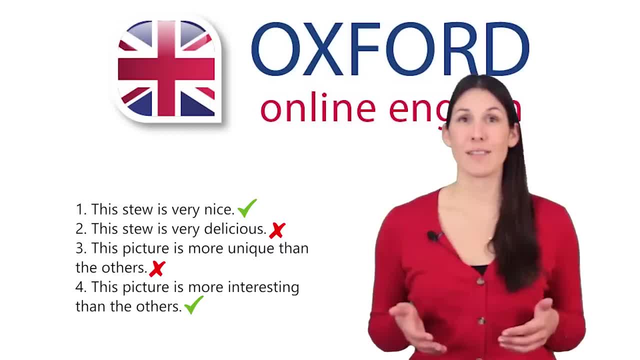 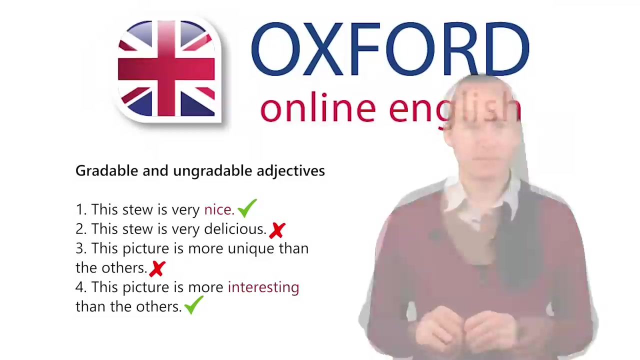 To explain this, you need to know about an important idea – gradability. Some adjectives are gradable. That means they can have different levels. For example, Nice and interesting are gradable. Something can be more interesting or less interesting. There are different levels of interesting. 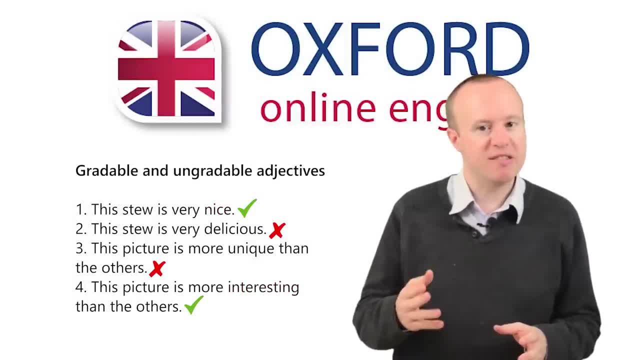 Some adjectives are ungradable. That means they're binary: either yes or no. For example, Unique is ungradable. Either something is unique or it isn't. You can't have different levels of uniqueness – it's a yes or no property. 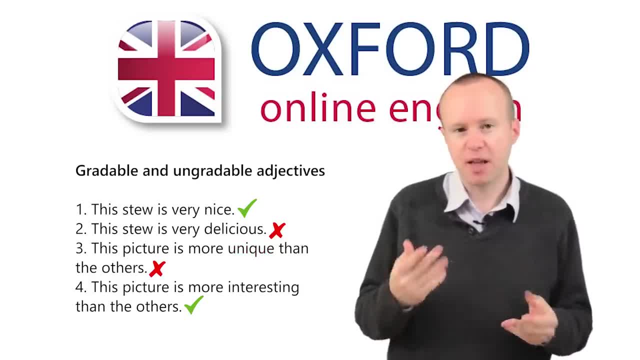 Ungradable adjectives have two types. Firstly, there are words with a strong meaning, like delicious, exhausted or furious. Secondly, there are words with an absolute meaning, like unique, true or possible. When we talk about ungradable adjectives, we mean both of these types. 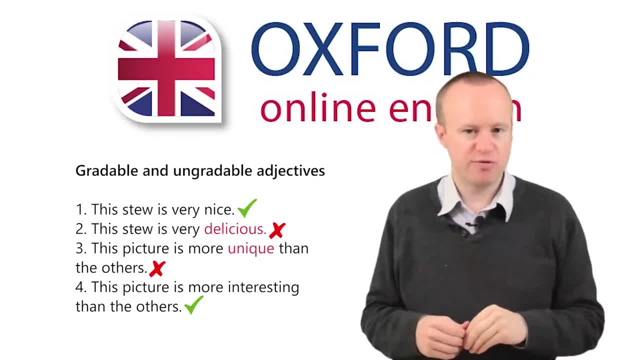 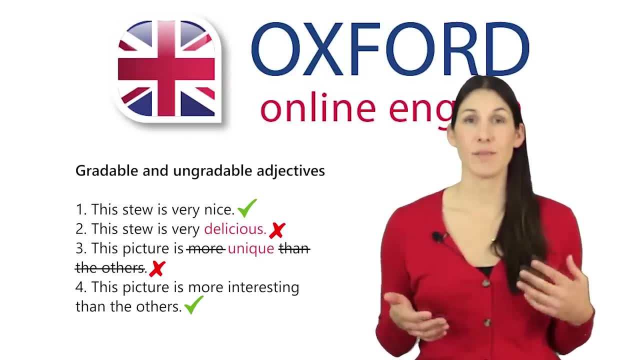 What does this mean for you? Well, there are two important rules you should know: 1. First, you can't make comparatives from ungradable adjectives. You can't say more delicious. You can't say truer or most possible. 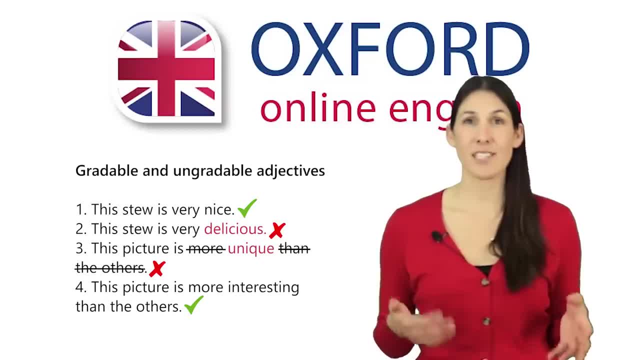 Secondly, if you want to emphasize an adjective by adding a word like very, really or absolutely before it, you need to use different words for gradable and ungradable adjectives. 2. Very is used with gradable adjectives, So you can say very big. 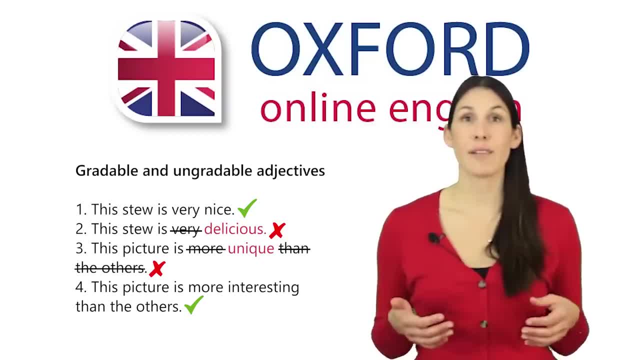 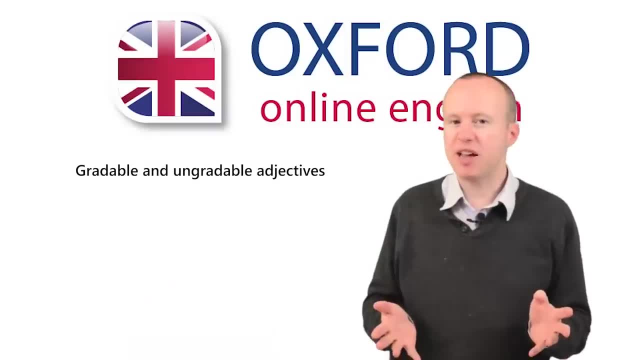 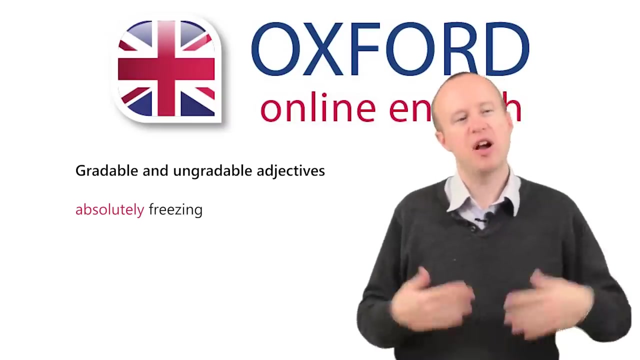 Very beautiful, Very cold Or very funny, But you can't say very gorgeous, very freezing or very hilarious. You can't say very freezing. But what can you say With ungradable adjectives? use absolutely. You can say absolutely freezing, absolutely exhausted or absolutely unique. 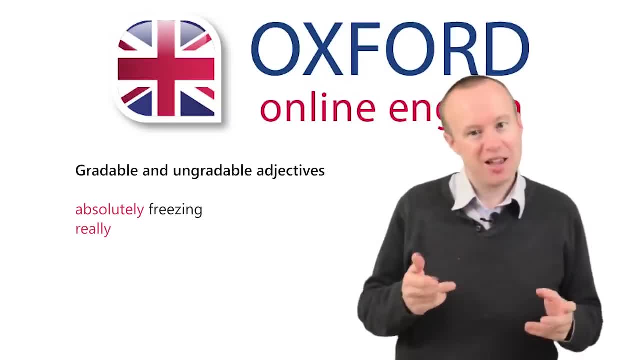 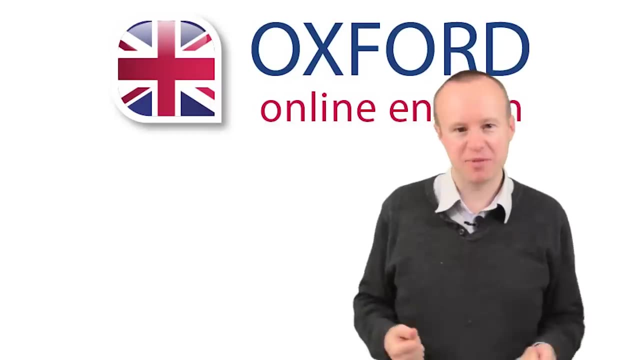 What if you're not sure? Use really, which can be used with both gradable and ungradable adjectives, So you can say really cold or really freezing, They're both fine. Understanding the difference between gradable and ungradable adjectives is important if 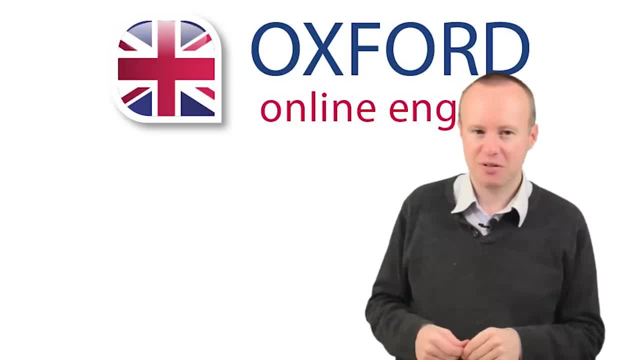 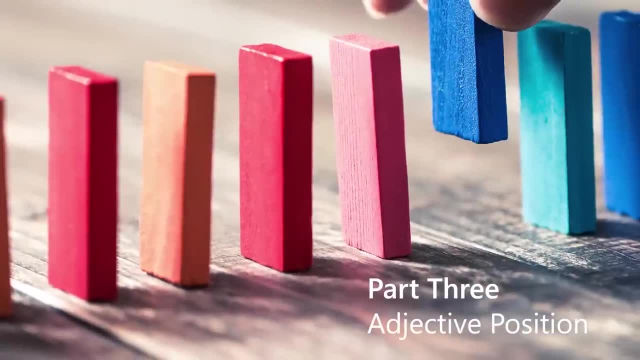 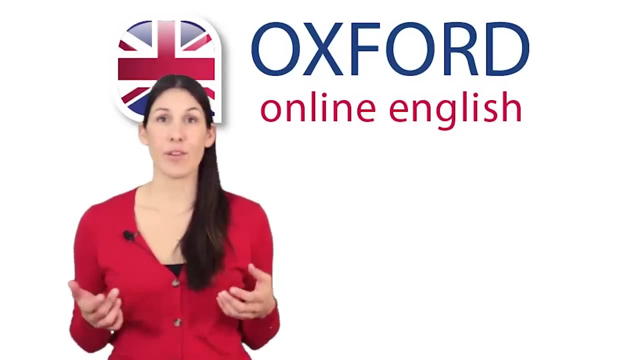 you want to use adjectives correctly in English. There's also one more important point you should know. Let's look: 1. You heard in part 1 that adjectives can go before the noun or after the noun if you use a linking verb. 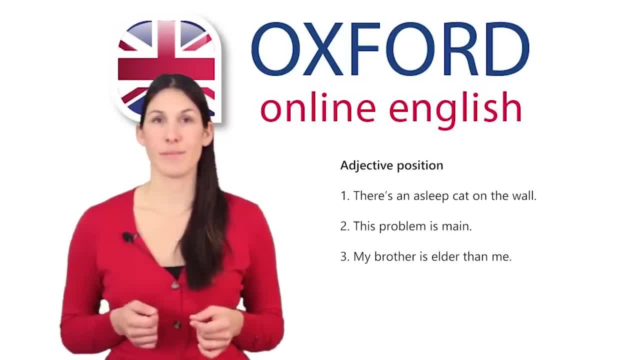 So are these sentences correct or not? As always, pause the video if you want to think about it for longer. Ready. Here's the answer. All three sentences are incorrect. None of them are possible. Do you know why? 2. 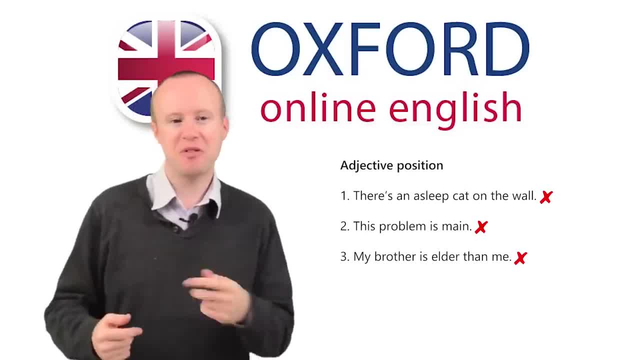 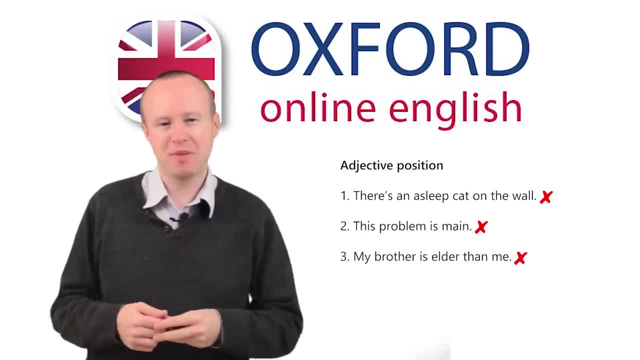 Many adjectives can be used either before or after the noun they describe. For example, you can say the car is new or the new car. Both are possible and it doesn't change the meaning. However, some adjectives can only be used in one position, either before or after the. 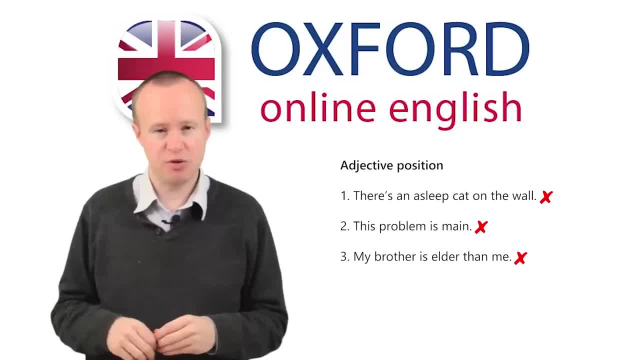 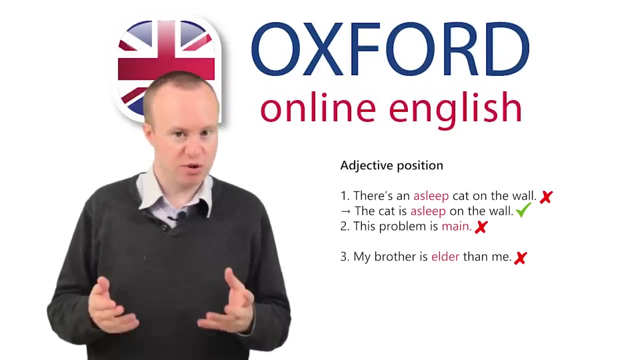 noun. That's the problem with the three sentences you saw just now. 3. Sleep can only be used after the noun it describes. You can say the cat is asleep on the wall, but you can't say an asleep cat. Main and elder are examples of adjectives which can only go before the noun. so you 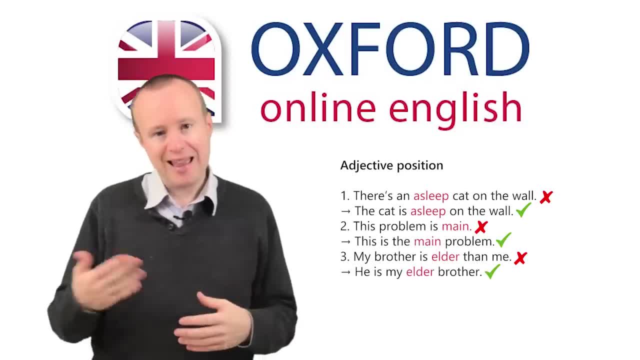 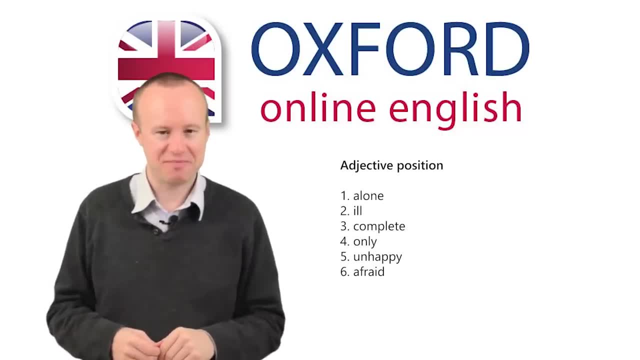 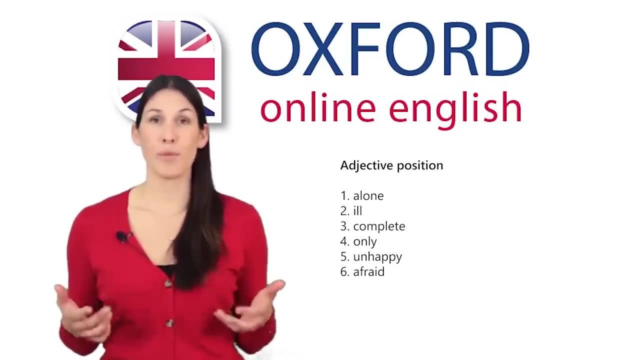 could say: this is the main problem, or he is my elder brother. Now let's do a test. Look at six adjectives. Here's the question: Can these adjectives be used before the noun, after the noun or in both positions? 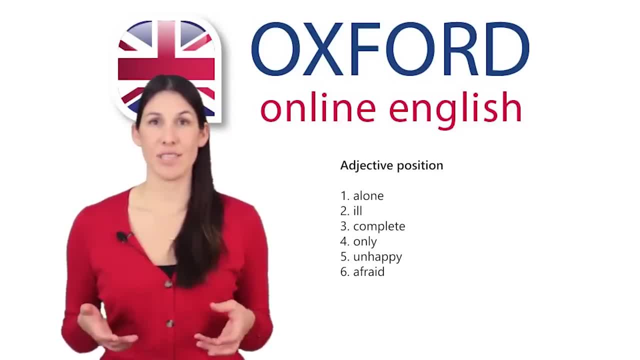 To do this, try making sentences with the six adjectives, or go to an online dictionary such as the Cambridge Dictionary or Longman and find example sentences. When you make sentences, try saying them out loud. Use your instinct. Does it sound strange or wrong? 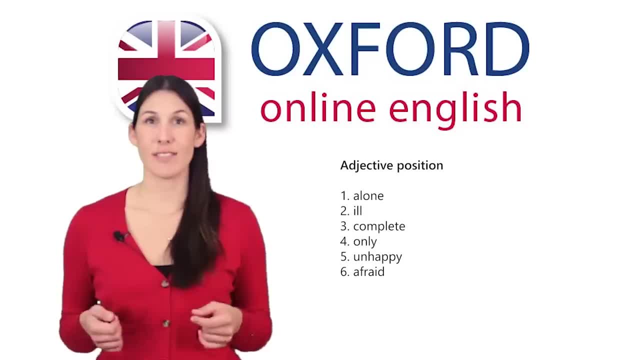 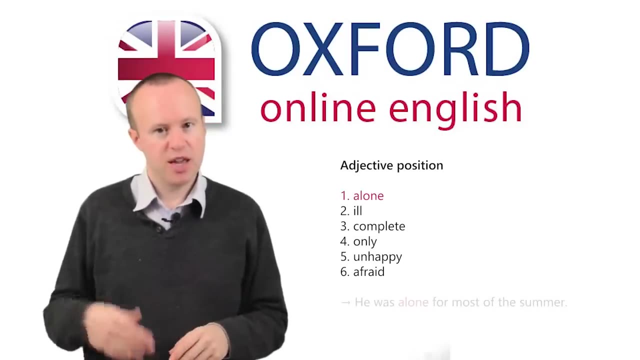 It probably is. Pause the video and do the test. You'll see the answers in a few seconds. Ready, Let's check together. Alone can only be used after the noun it describes. For example, he was alone for most of the summer. 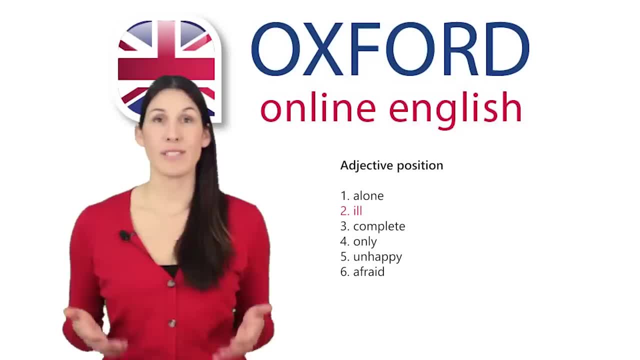 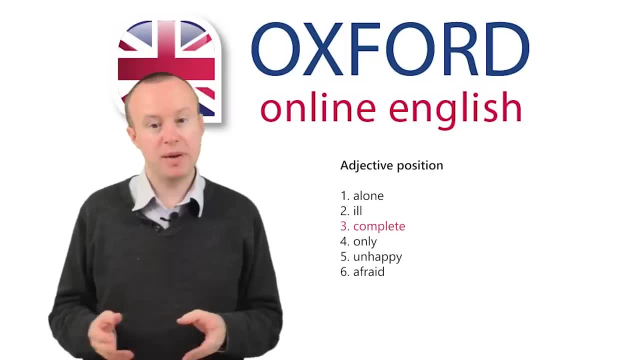 Ill is also generally used after the noun it describes. For example, I didn't work yesterday because my daughter was ill. That's a use too. Listen carefully to this and you'll understand what I'm talking about. 3. COMPLETE can be used in both positions. 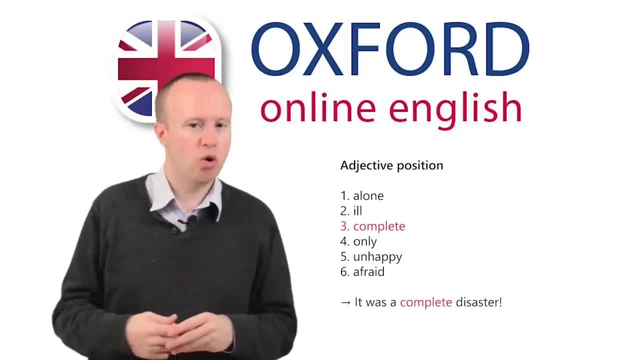 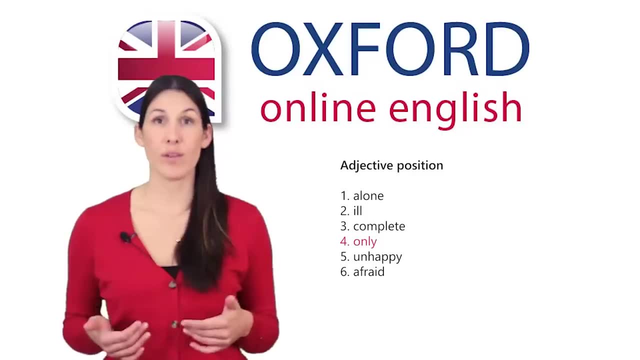 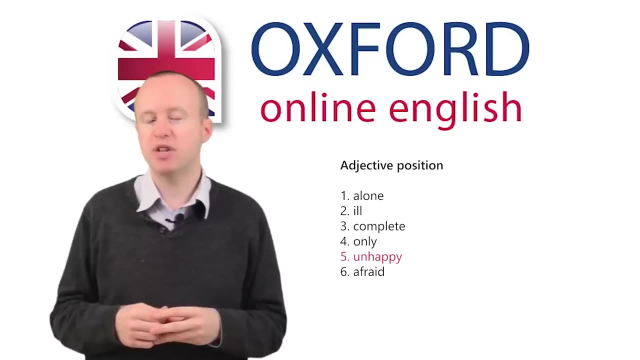 For example, it was a complete disaster or the first stage of the work is now complete. ONLY is used before the noun, For example, the only way to do it is to do it yourself. UNHAPPY can be used in both positions. 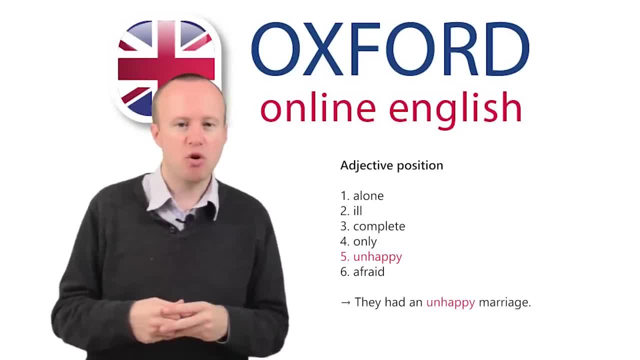 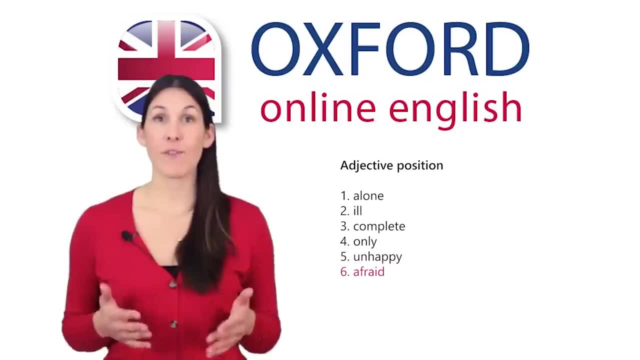 For example, they had an unhappy marriage or he didn't enjoy the last year of school and was often unhappy. Finally, AFRAID is only used after the noun. For example, I was afraid of the dark when I was a child. 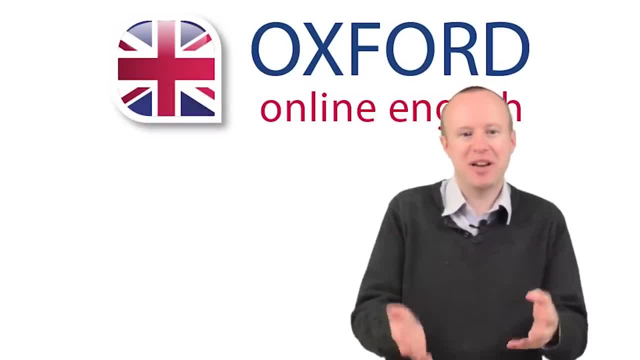 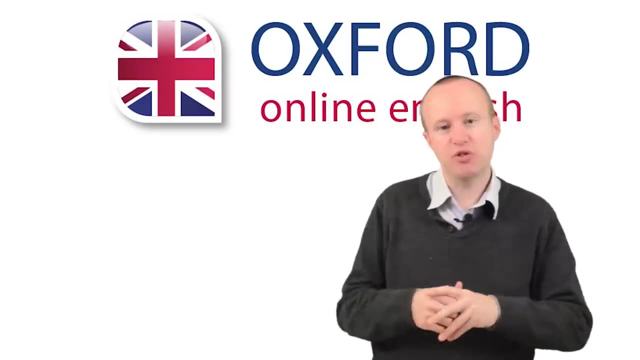 So you're probably thinking: how do I know? How do I know whether an adjective can be used before or after a noun? It's a good question. Unfortunately, there isn't a simple answer. Dictionaries don't usually include this information. 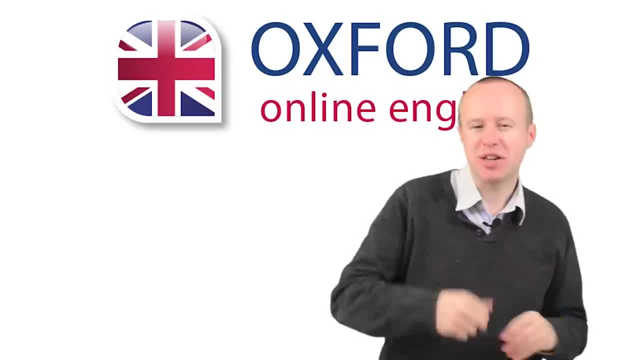 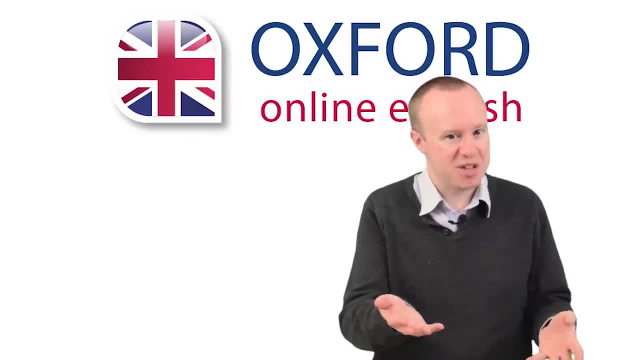 However, we have good news. Most adjectives can be used in both positions. Also, for most adjectives which can't you already know the answer, For example, remember the sentence. the problem is main. Most of you knew that this sentence sounded wrong. 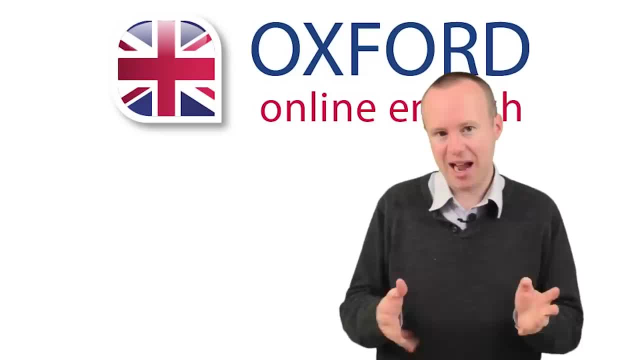 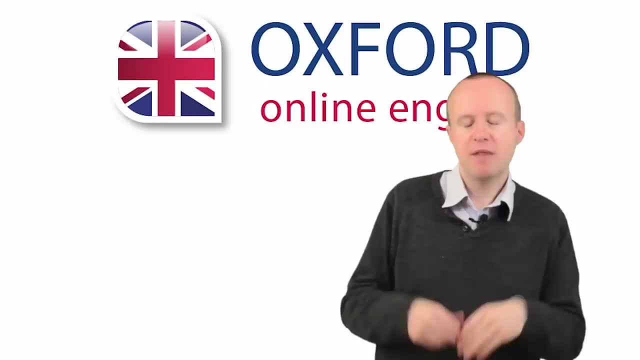 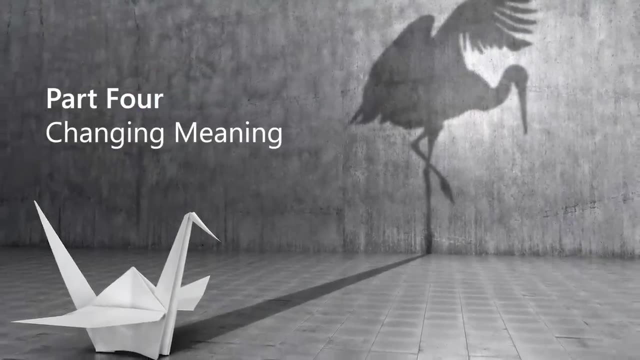 Your instincts can be helpful. Anyhow, now you know about gradability and adjective position. there's a reason we've shown you these two topics, because our last idea depends on these points. You know that adjectives can be gradable or ungradable, or that they can go before. 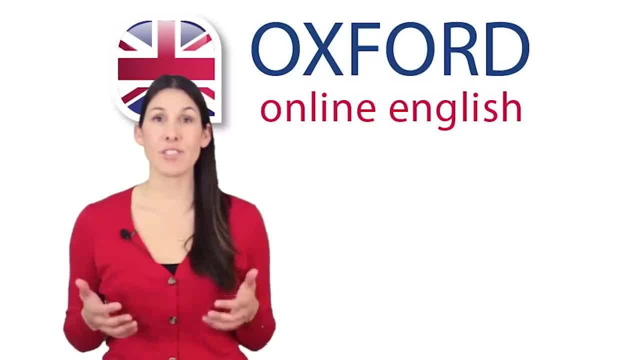 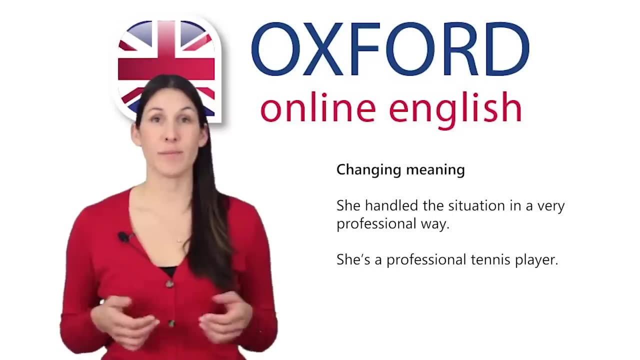 or after the noun, but in some cases the same adjective can be used in different ways, with different meanings. For example, look at these two sentences. She handled the situation in a very professional way. She's a professional tennis player. Both these sentences use the adjective professional, but in different ways. 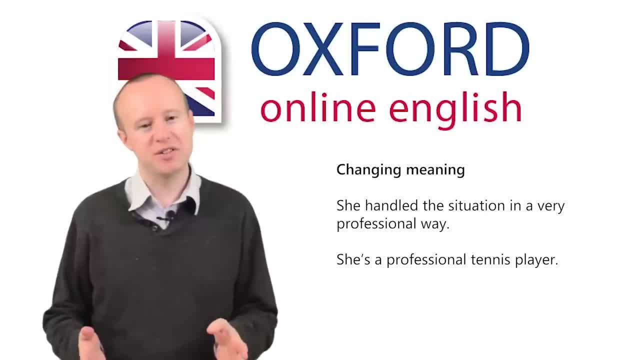 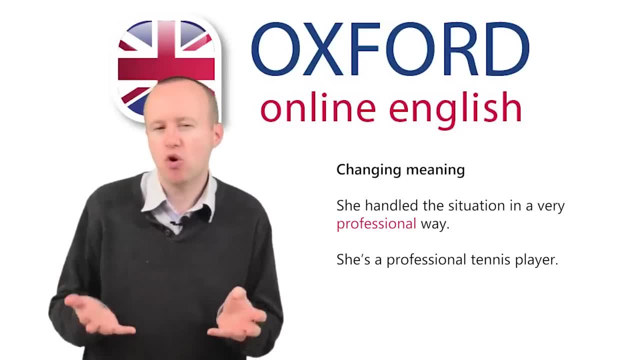 Can you see the difference? In the first sentence, professional is used as a gradable adjective and it means something like effective or competent. In the second sentence, professional is ungradable. It means that playing tennis is her job and she makes money from it. 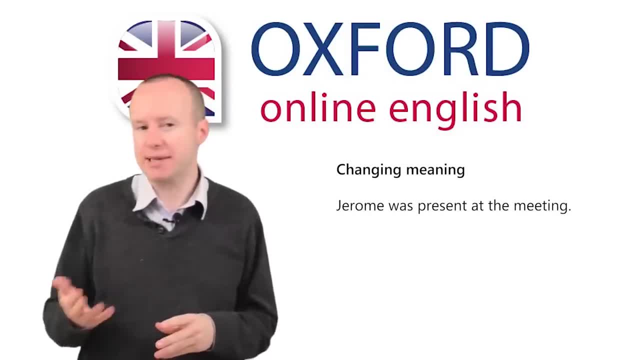 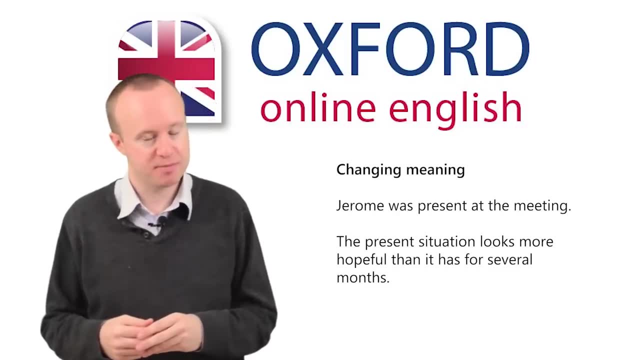 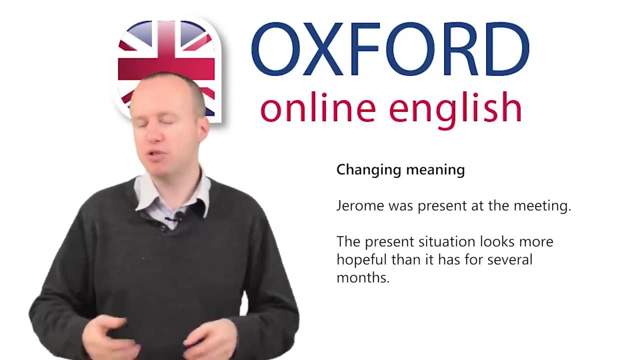 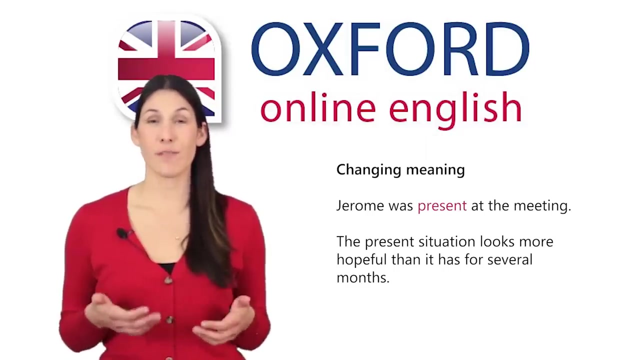 Let's do another example. Jerome was present at the meeting. The present situation looks more hopeful than it has for several months. What about here? Can you explain the difference between these two uses of present? In the first sentence, present is used after the noun with the linking verb. 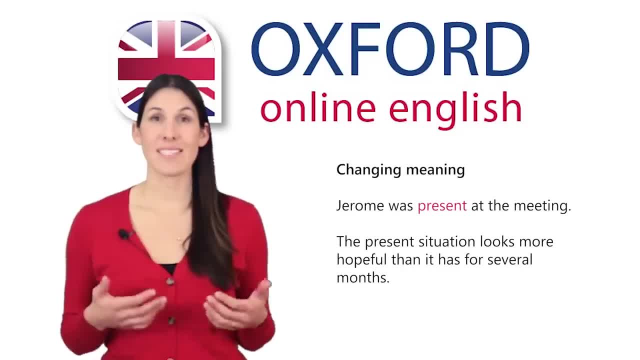 It means that Jerome was there. In the second sentence, present is used before the noun and it means relating to now. So in this case the adjective has different meanings in different positions. To be clear, this isn't flexible. You can't choose to use present before a noun to mean there. 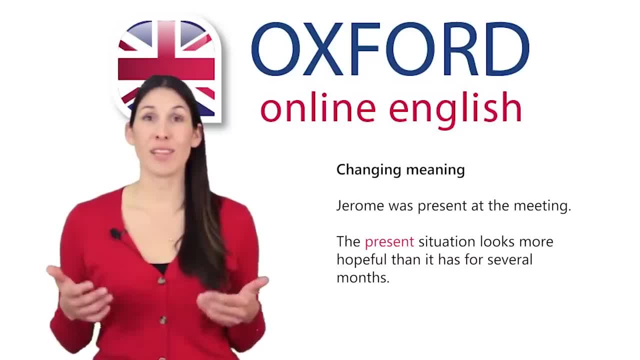 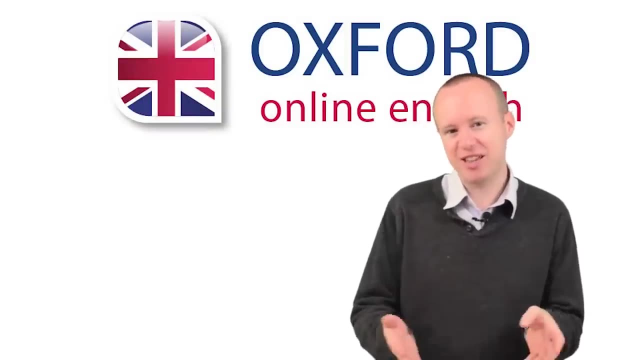 If you use present before a noun, then it means relating to now. So what should you take away from this? What do you need to focus on? We aren't showing you these points because you need to learn lists of all the gradable and ungradable adjectives. 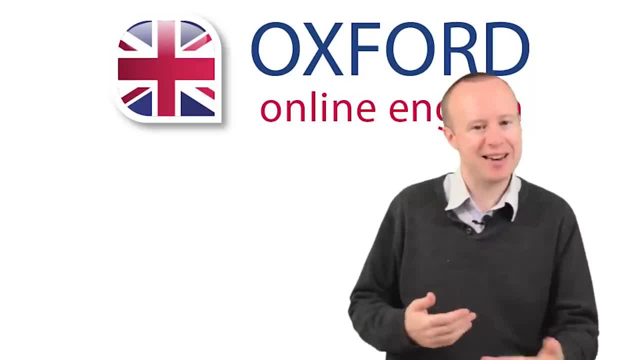 This lesson gives you tools to help you understand adjectives more deeply. The most important point is that adjectives don't follow one simple set of rules. Like with all vocabulary, you need to use context to understand what an adjective means in a sentence. 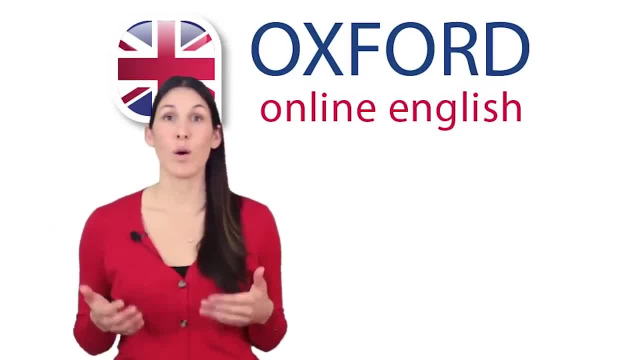 Next, and this is also a general point, one word doesn't have one meaning With adjectives. whether a word is gradable or not can make a difference. Where an adjective is used can make a difference. You can't simply rely on a dictionary or a translator.